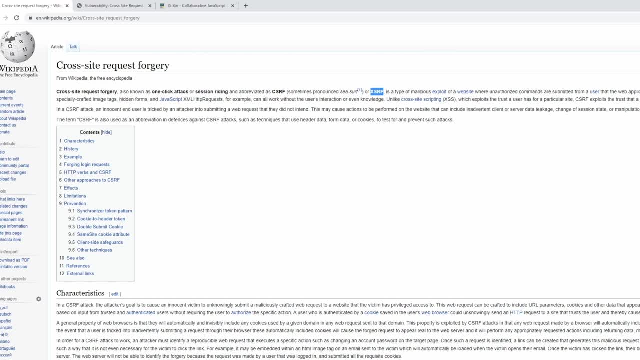 session writing or XSRF. Generally speaking, if you're looking for any type of literature that's serious on cross-site request forgery, for example, if you're looking for like an actual cross-site request forgery, you can look at the one-click attack, which is a one-click. 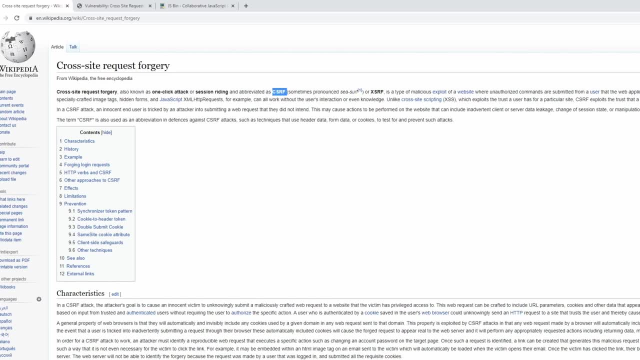 attack and you can look at the one-click attack, which is a one-click attack, which is a one-click paper. You'll see it either spelled out like this or written as CSRF. So what is a CSRF attack? Well, a CSRF attack is an attack in which a end user- so let's just say: 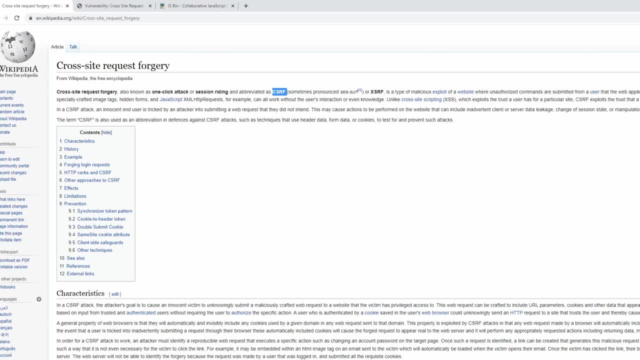 you're logged into your YouTube account, you own that YouTube account and there's a relationship between you and YouTube where you pass back some identifiers with each request and, as a result of that, YouTube knows that you're privileged and allows you to do operations like, for example, uploading new videos, deleting existing videos, changing your 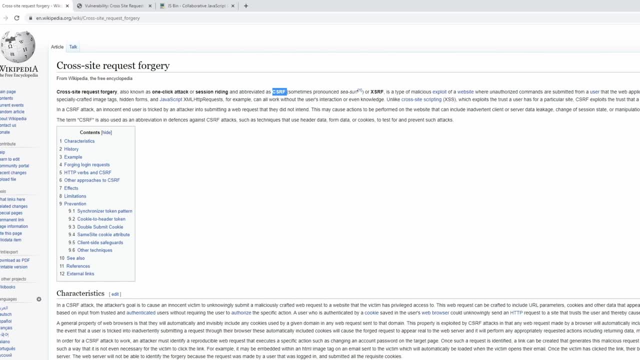 avatar, etc. now you can do that because you have this privileged relationship with your youtube account. you've proven who you are now. a hacker or another malicious actor that does not have access to your youtube account would not be able to upload videos on your behalf. delete videos on. 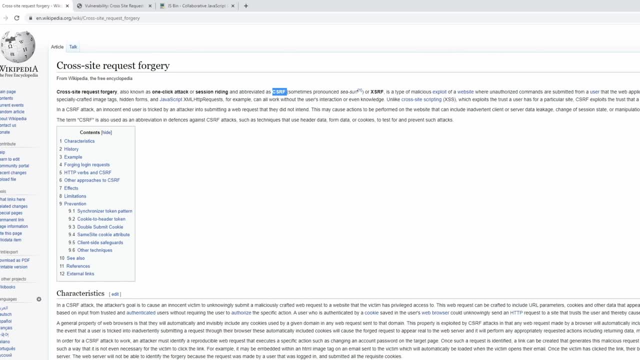 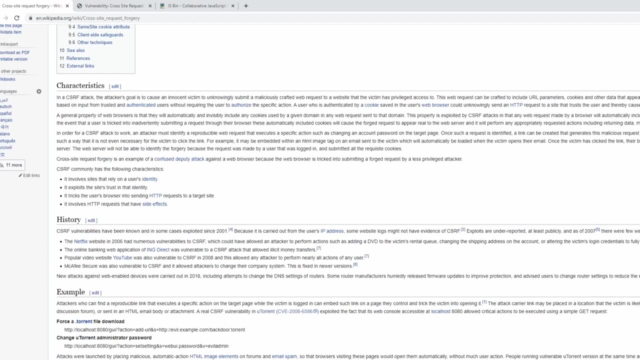 your behalf or change your avatar. so what they might do is try to find a way to get your browser to trick youtube into thinking a request is coming on behalf of you, the account owner, when in reality that request is coming on behalf of a malicious user, and you can see in the wikipedia page here: 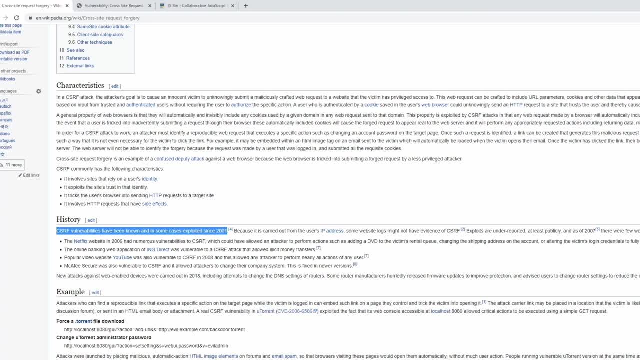 that c-ser vulnerabilities are nothing new and, unfortunately, they're very widespread. you can see that netflix has been vulnerable to c-serve attacks, various banking applications, youtube was vulnerable to c-serve attacks in 2008 and this allowed an attacker to perform almost any action. 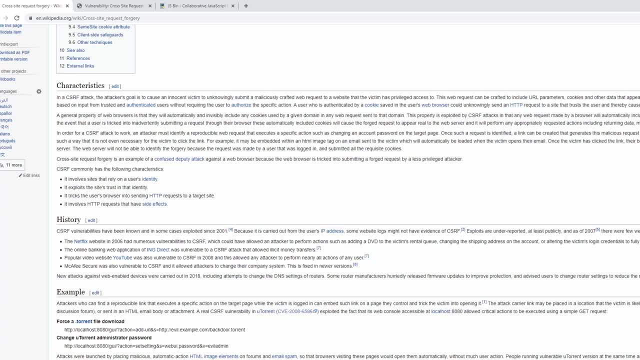 on the internet and YouTube allowed an attacker to perform almost any action on the internet to a user. fortunately, that has been patched. even mcafee secure was vulnerable to csurf. a business that claims to build on top of their reputation for security was vulnerable to csurf attacks. 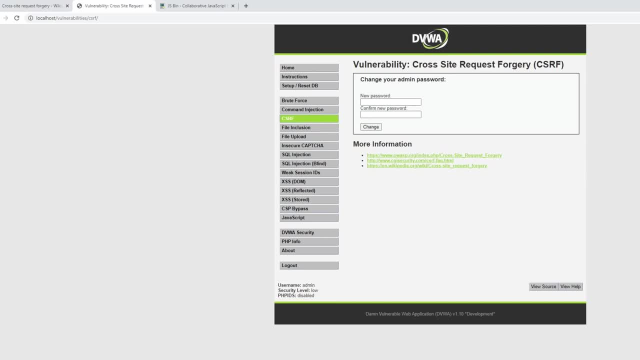 well, let's demonstrate a csurf attack and maybe it will become a little bit more clear. so this is dvwa, aka damn vulnerable web application, version 1.10. so this is an application that is, on purpose, full of security vulnerabilities, for the sake of education, for the sake of testing. 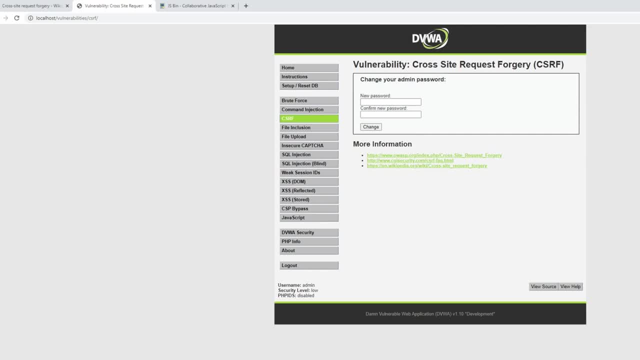 etc. and i'm using this application to demonstrate a simple csurf attack. so on this page you can see that there is a form field that allows you to change your admin password. so let's try changing our password to test. when we click change, a network request occurs and it says password. 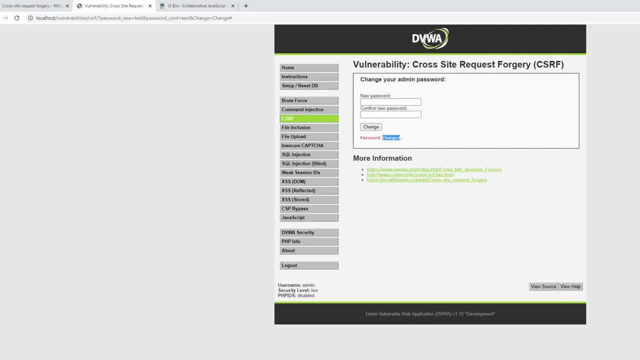 changed. we don't even have to go to the network tab to know what network request occurred, because we can look up here and we can see that we're at localhost vulnerability csurf. so that's the tab right here. but then after the question mark there is a query. 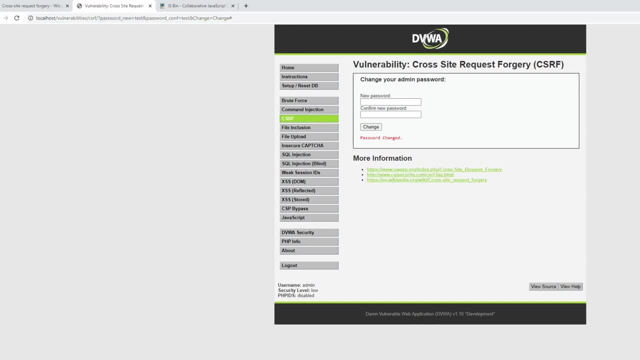 parameter password underscore: new equals test. so what's going on here is that there's this thing called http, and this is a method of sending information over the web that browsers have chosen to adopt. it's a protocol, and http has these verbs, which are different ways of interacting with. 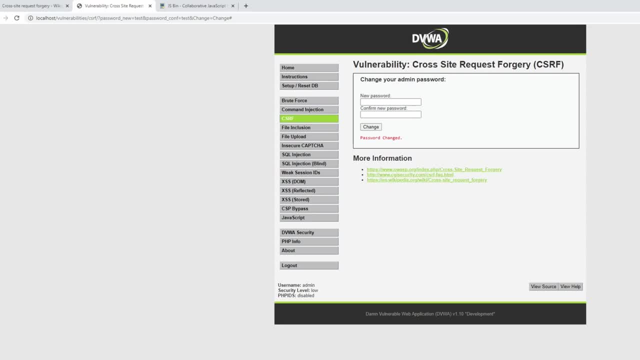 servers. the dvwa, aka damn door-to-door service, is your only available service so you can go to the or the most commonly used one is called a HTTP GET request. So whenever you see a hyperlink, for example, the majority of these are hyperlinks- what's going on? 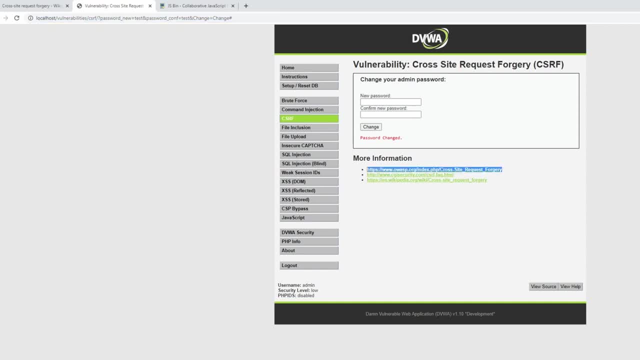 behind the scenes is you click on a link, you'll see this one. right here is a hyperlink that goes to OWASP, OWASPorg, slash index, etc. So when you click on a hyperlink, any hyperlink, your browser is going to perform an HTTP GET request. 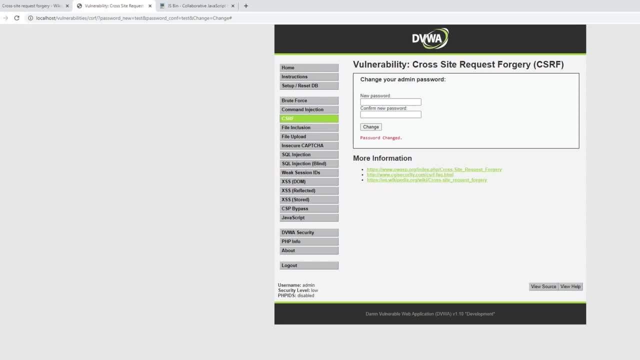 using the HTTP protocol and the GET verb, and that is a specific methodology for talking with a server. That methodology allows you to pass back query programs. Generally speaking, GET requests are intended to be used for retrieving information. When you start to use them for setting or modifying, 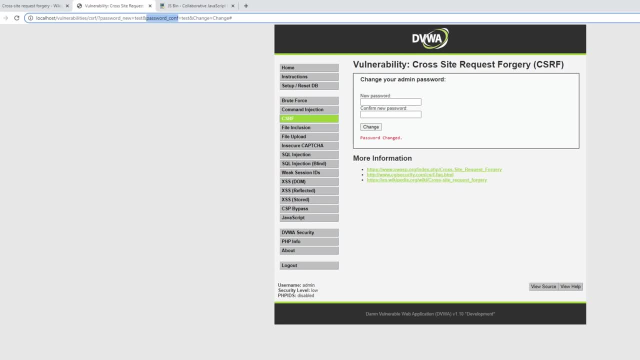 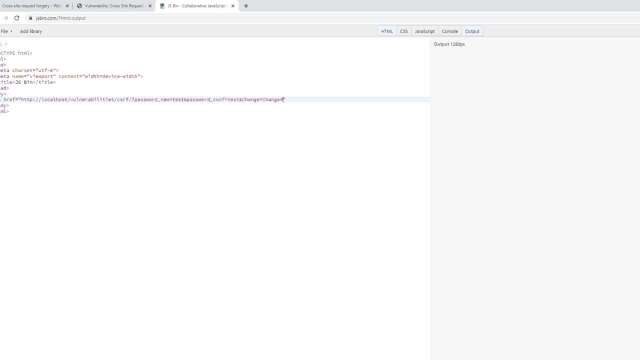 information. that's when you run into some issues, So let's just go with this fact that this URL is capable of changing state. So here I am in jsbin, an application that allows you to create arbitrary JavaScript and HTML websites for the sake of testing. Now, because 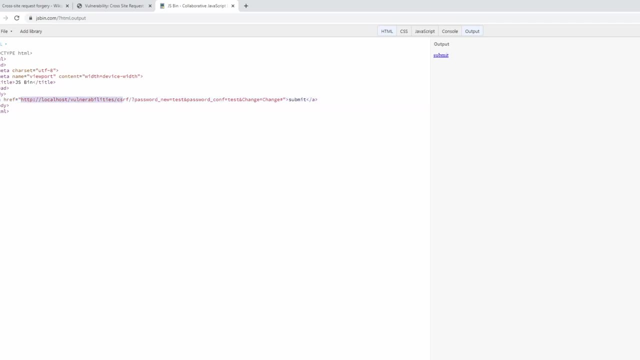 HTTP GET is the language of hyperlink. if clicking on this link changes your password, which we know it does, then password underscore new. the parameter here could be set to anything, So we could set it to, for example, test5.. And by clicking on this hyperlink you would. 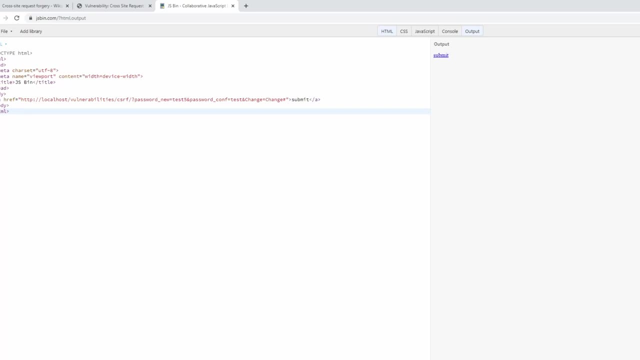 change the password of the currently signed in user. So how does this work in practice? So imagine a website is vulnerable to csrf attacks and the csrf attack is a state-changing GET request. Now what can happen is someone can distribute a hyperlink and trick you into clicking it. You'll see the 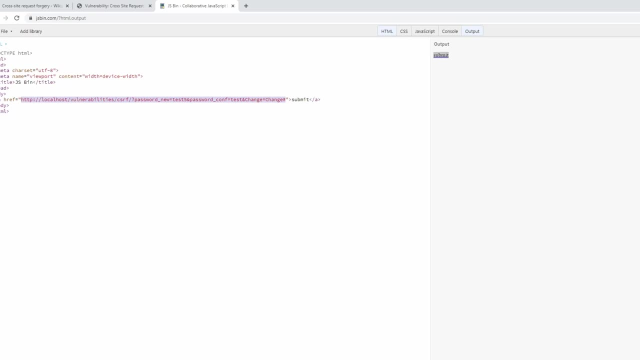 hyperlink here doesn't even have to say that it's pointing to this website. it can say anything the user wants. So you can. you can send them a link that appears as if it's going to Amazon. If they're not paying close attention when they click on it, it really goes back to 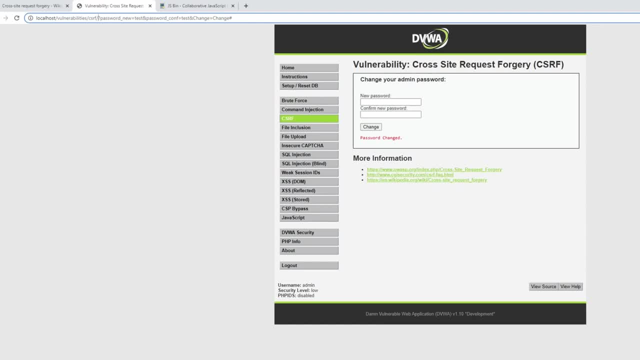 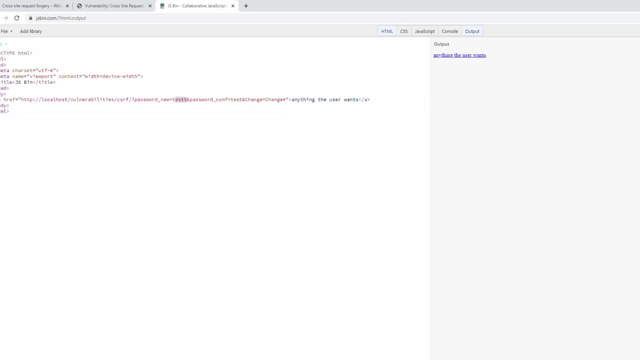 this web application and the server interprets it as: hey, we're doing a password change. Now, by clicking on that, your password has been changed to something that the malicious actor, aka the hacker, is aware of. He can log into your account and he can change things, etc. So state-changing GET requests are: 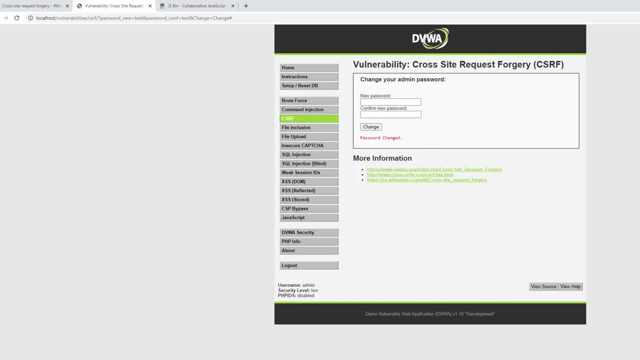 the most common form of csrf. Cool, so we can summarize this by saying: csrf attacks occur when your privileged relationship with a server is compromised because a malicious actor has found a way to convince your browser to make requests to that server on your behalf, as if it were coming from you. but it's actually coming from the malicious. 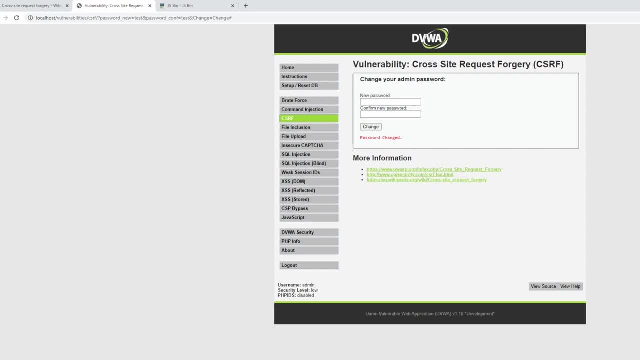 actor who either convinced you to initiate it or tricked you somehow, or tricked the browser. One of the most common mitigation you'll see is to use POST requests, because the HTTP GET obviously can be clicked on, but another verb, HTTP POST. you have to include parameters in. 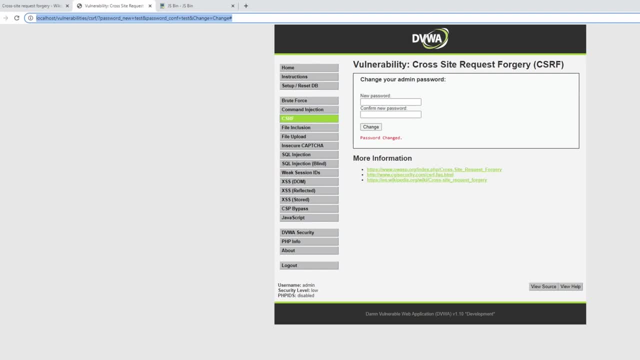 the body And the web browser does make it a little bit harder to initiate HTTP POST requests on behalf of a user, but it's not very hard. For example, a web form like this on another page could point back to the server, the API that 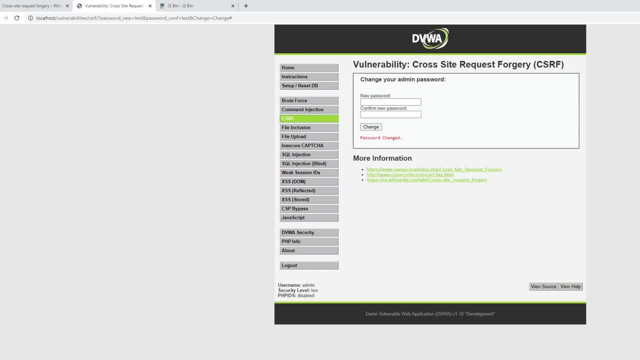 powers. this website And web forms by default initiate HTTP POST requests. So ultimately, there's a number of mitigations people think work and there's some that may work conditionally, But if you're trying to protect against csrf attacks, the only or the best proven way that you can do this is each time.